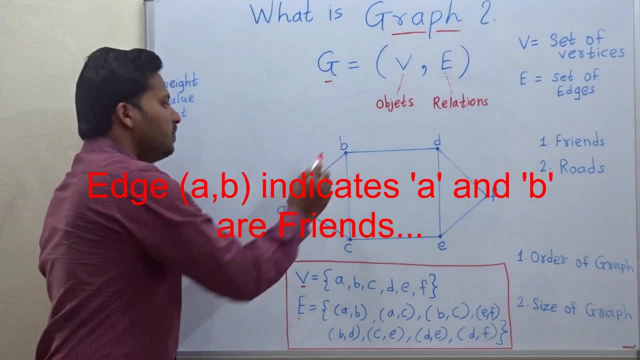 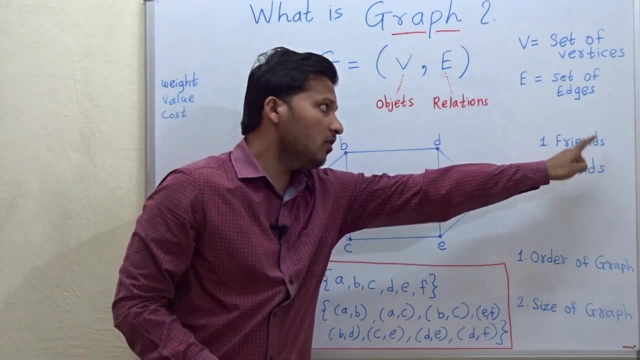 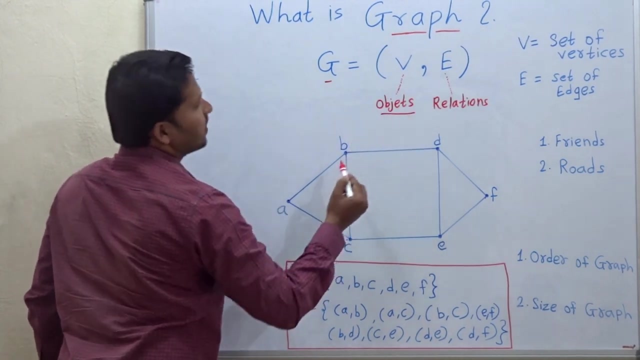 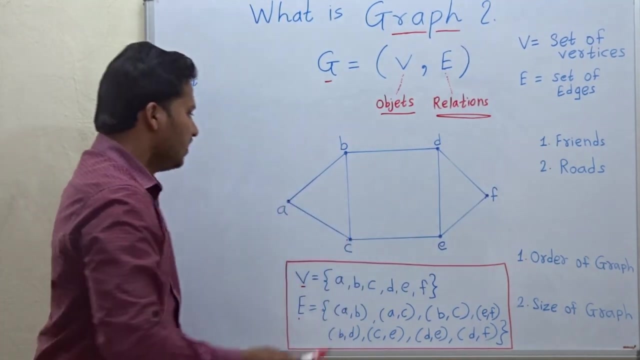 in A and B. So this edge A- B indicates that A and B are friends. The example is for friends and friends. Friends relation means these vertices are the objects and the edges in those vertices are the relations. So friendship is a relation. So person A and person B are friends. but there 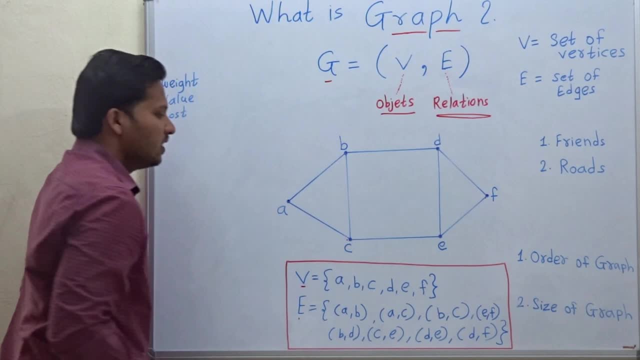 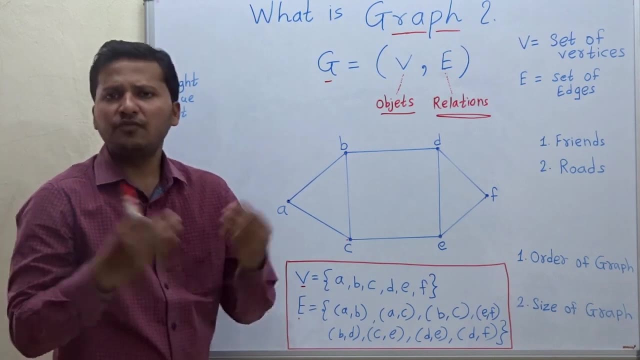 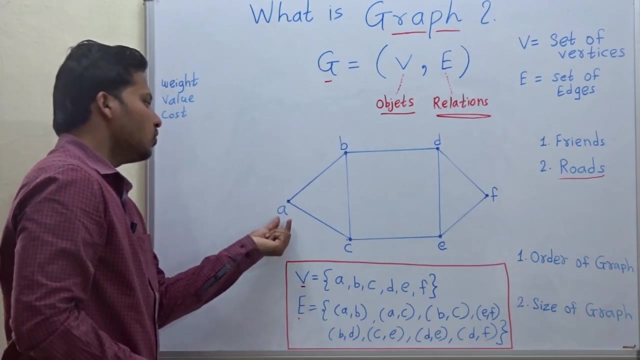 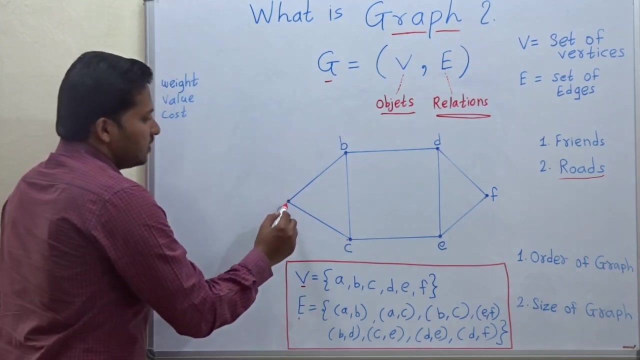 is no edge between A and F. So that means A and F are not direct friends. or you can say that A and B are not friends. Now let take another example of roads. So suppose A, B, C, D, E, F are the names of cities, So the 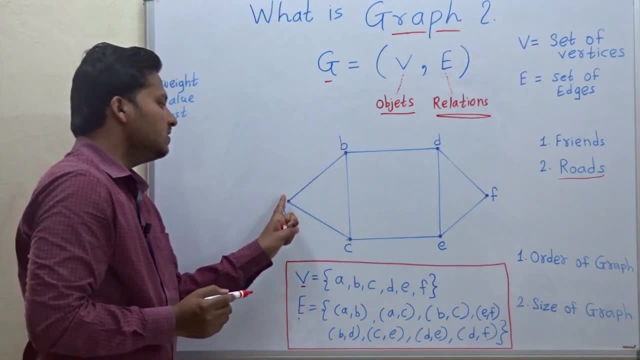 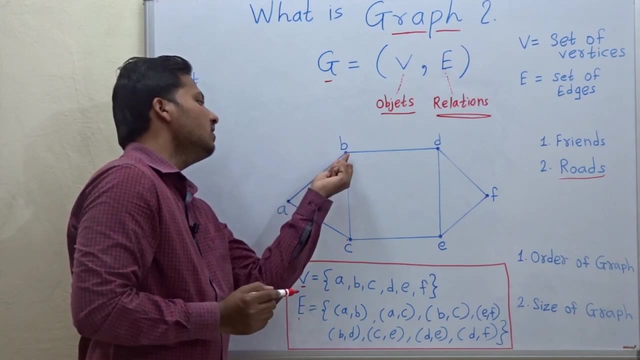 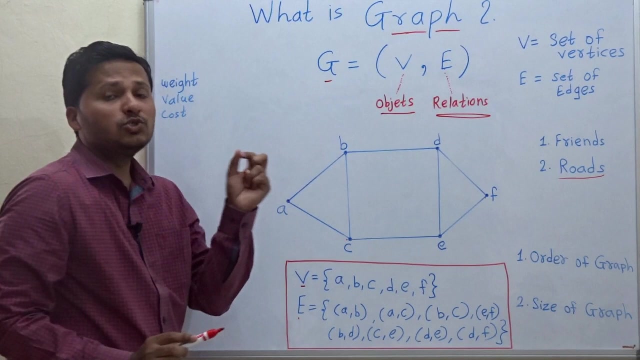 edge between A and B tells us that there is a road available between A and B means there is a direct road between city A to city B, But there is no edge between A and B. So the edge between A and F means there is no direct road between A and F here. Okay, so this is the 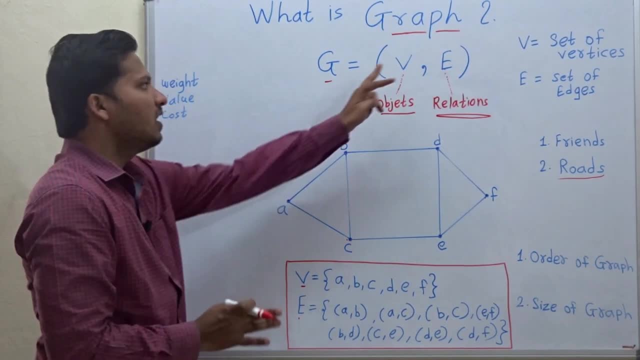 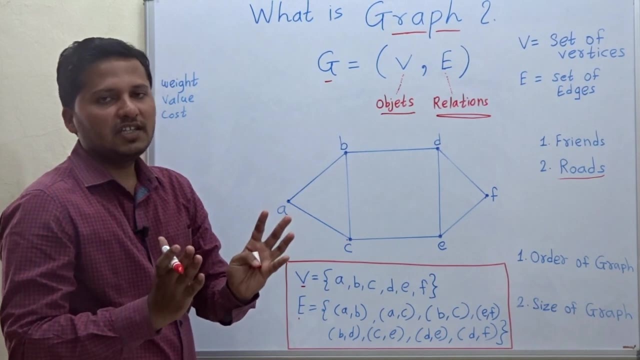 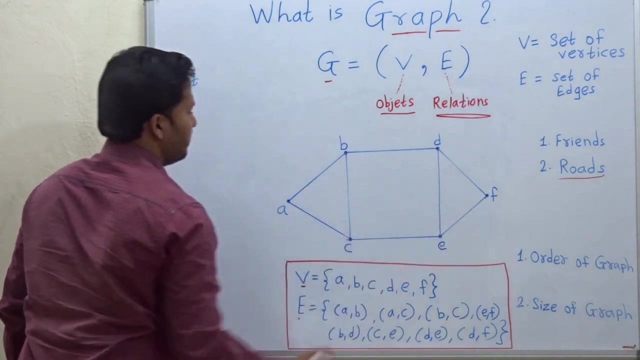 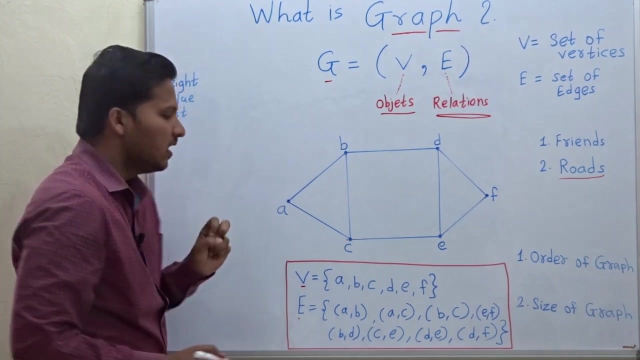 meaning of graph in the real world means the vertices are the objects and the edges indicate the relation between those vertices. So now these edges can also have some values associated with them. So, as you can see, A and B are cities. We have assumed that these are the cities. Then the 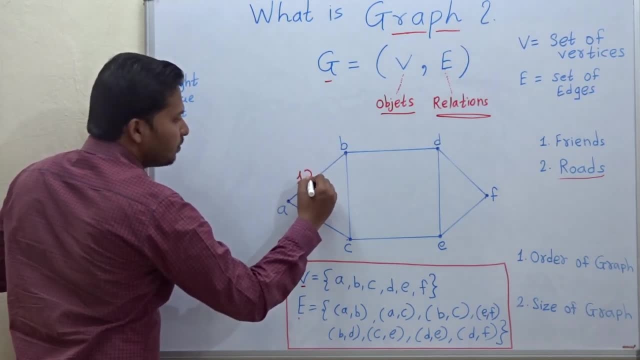 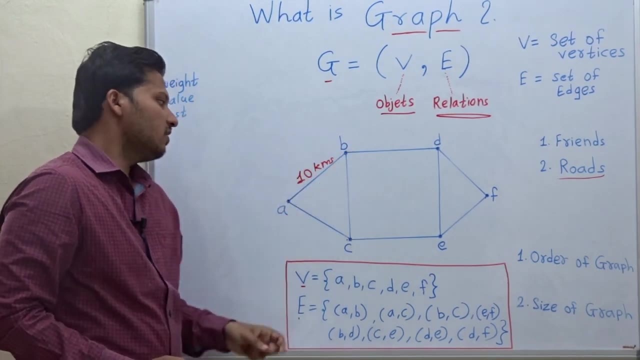 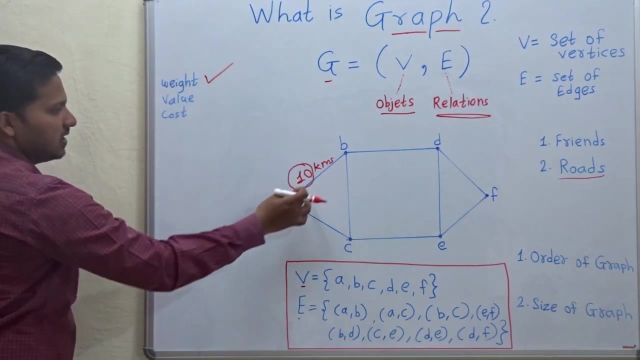 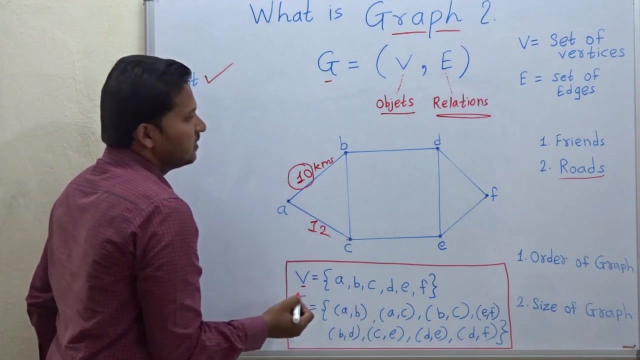 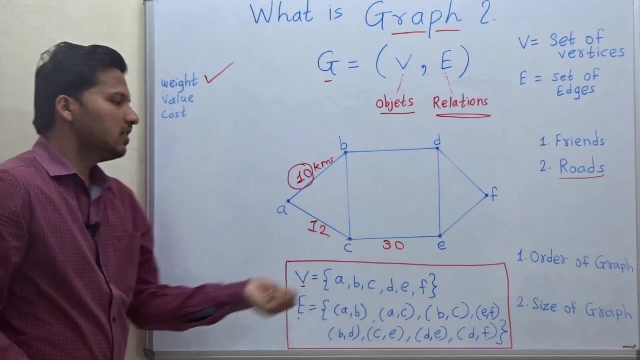 edge AB may have value. suppose 10 kilometers means the distance between A and B city is 10 kilometer, So the value for this edge is 10.. You can say that the weight of this edge is 10.. Okay, then suppose the value for AC is 12.. Then the value for CE is 30. Okay, so this is the weight for those edges.